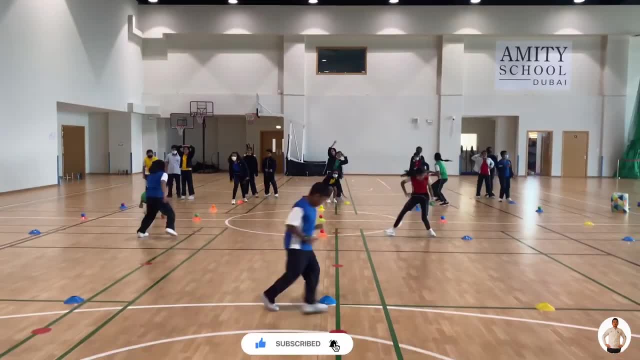 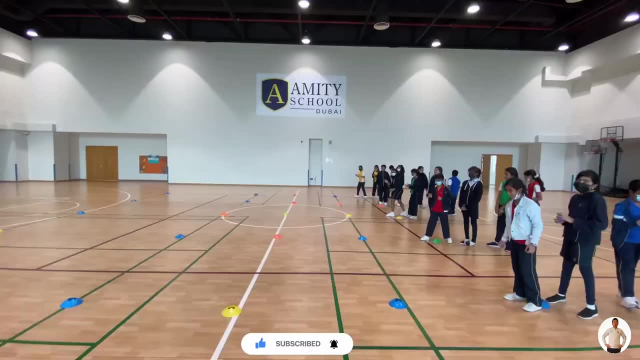 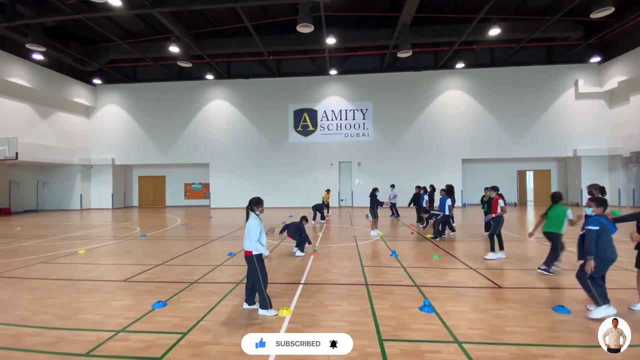 If they miss the catch, they cannot progress to the next marker, but the throwers will keep rotating. Once the catcher completes the second, last marker, they will run around the last one. Whichever team finishes first will be the winner. All the players get a chance to be the catcher. 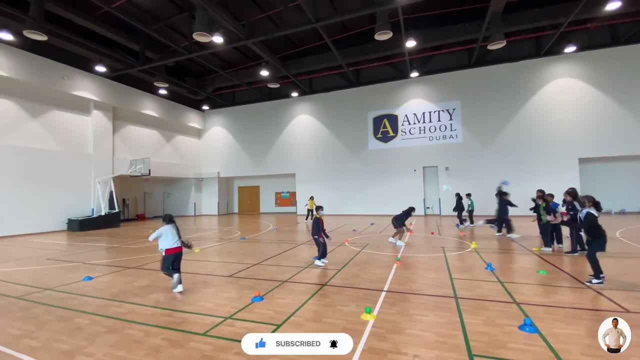 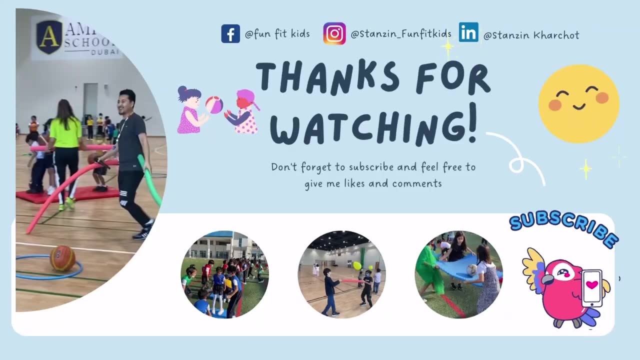 To make it easier, reduce the distance between each marker or use a bigger ball size. This is the end of the video. Thank you for watching. See you in the next video.